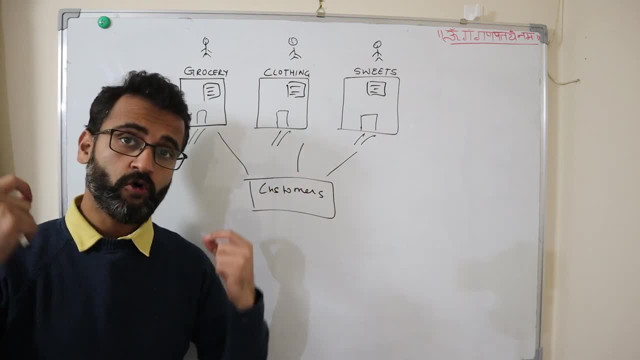 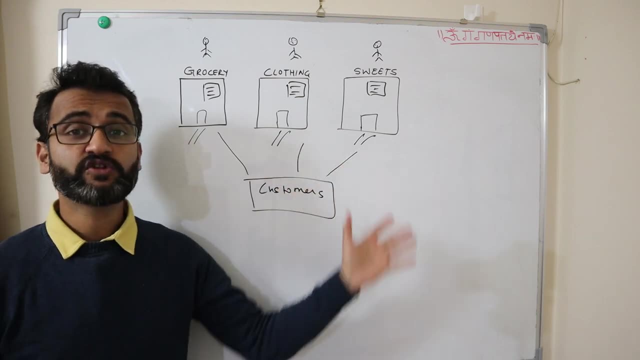 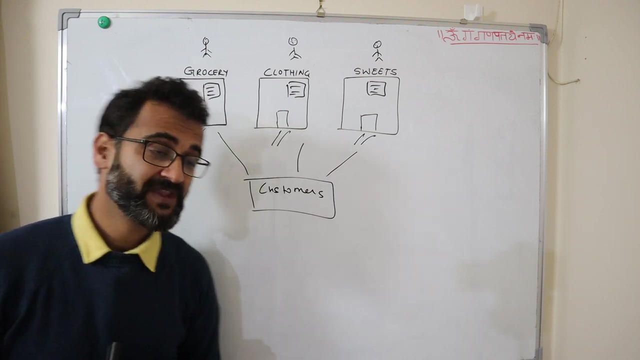 customers of all these three shops. So they wanted to give special offers to those customers who were literally coming buying grocery, buying clothes and sweets from all three brothers. So they wanted to get the list of all those customers from the village. But it was very 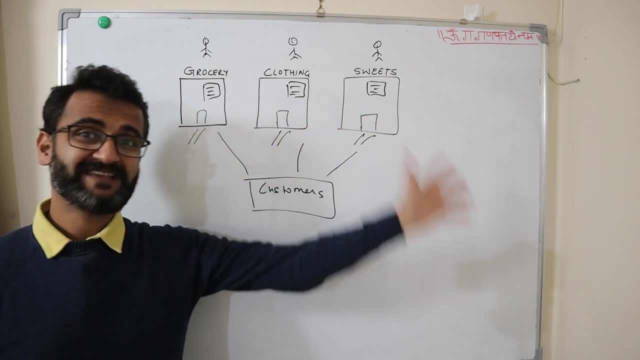 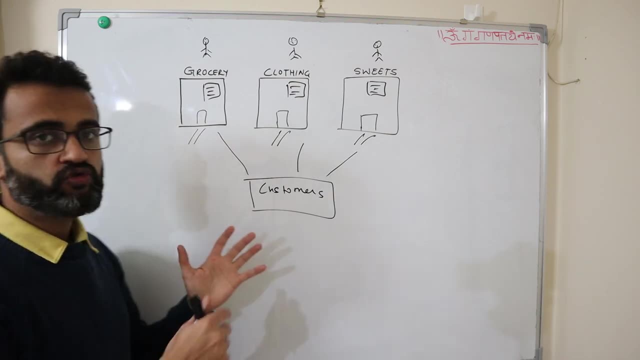 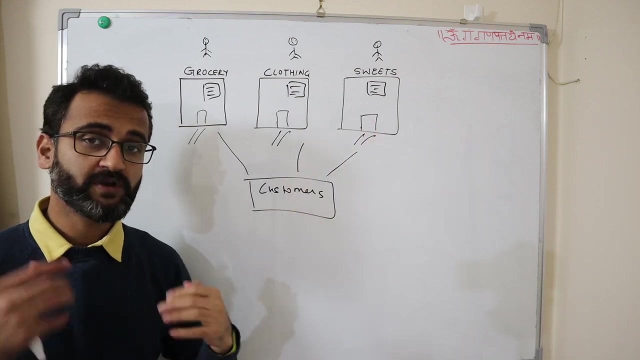 tedious because these three registers were maintained separately in individual shops And whenever they used to do this exercise at the end of the month, they used to combine this data, see the customer name and then match the data across various registers. So it was very, very slow. 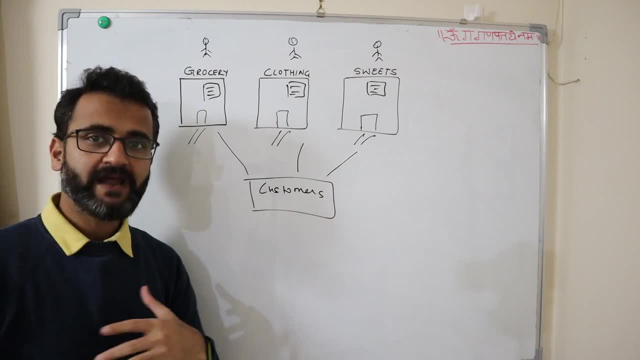 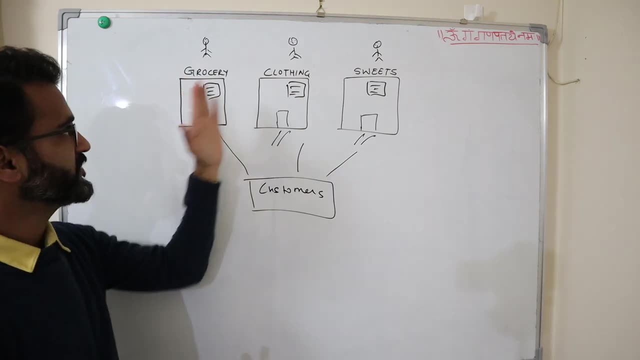 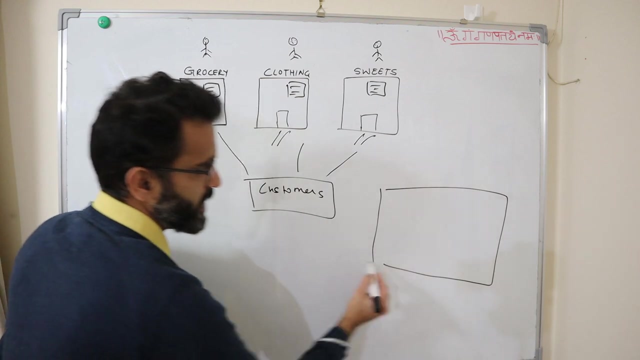 So they came out with an idea that, instead of having individual register, where they will have individual items to record for individual- you know- specific shops, they will have a combined register And this combined register will have data entered for all the three shops. 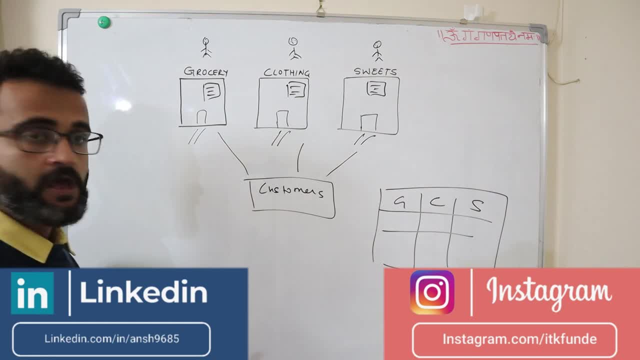 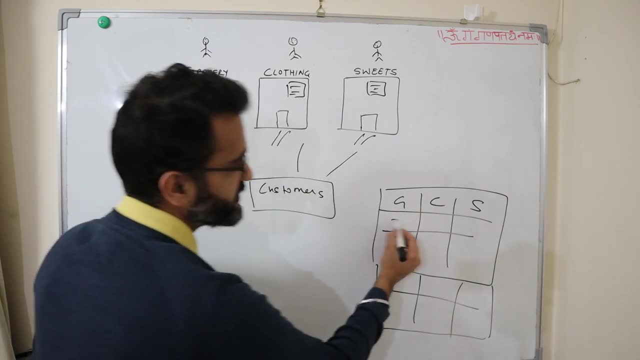 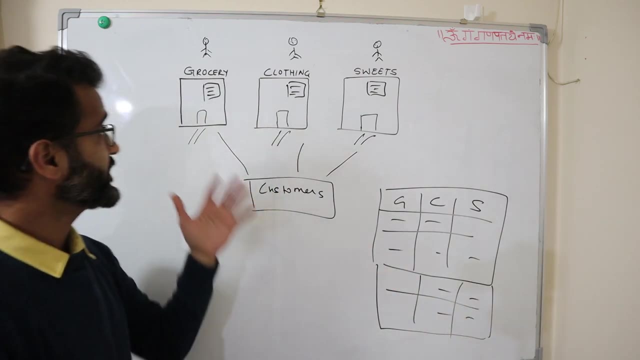 So grocery, clothing and sweets. Now this was a bigger register. This was way bigger than the ordinary register because here the entries were made for all the customers across all the three shops. So then there could be instances wherein you know a customer is coming and buying grocery, but you know he's not buying anything. 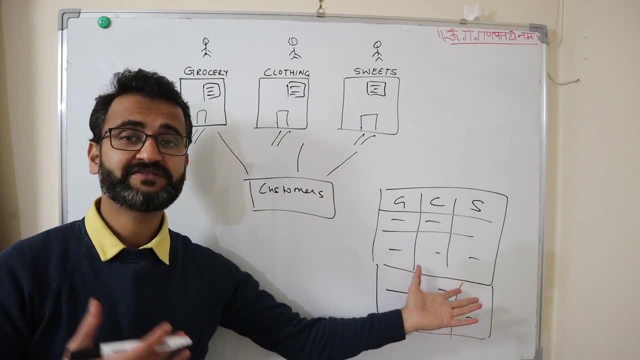 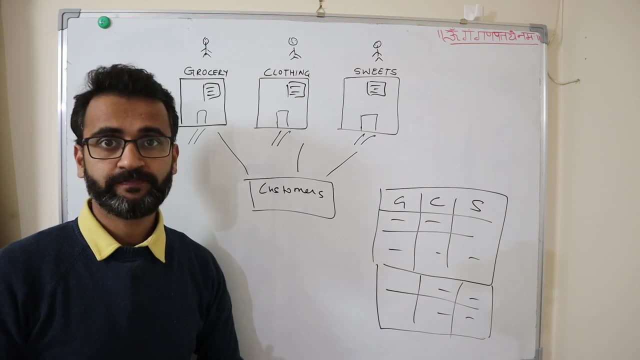 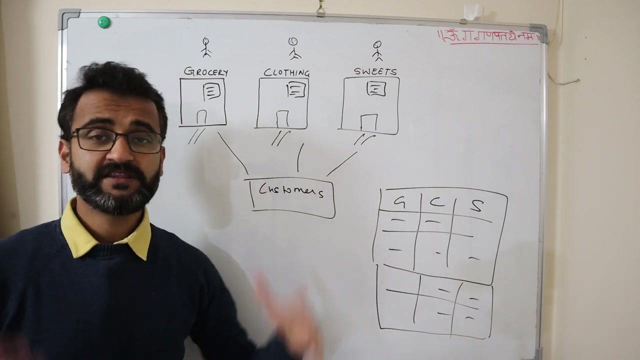 from the other two shops. So in that case you know the data, the register. just leave those- you know items blank for clothing and sweets and likewise for other shops also. No advantage of it was that when at the end of the month they used to see this register, they got all. 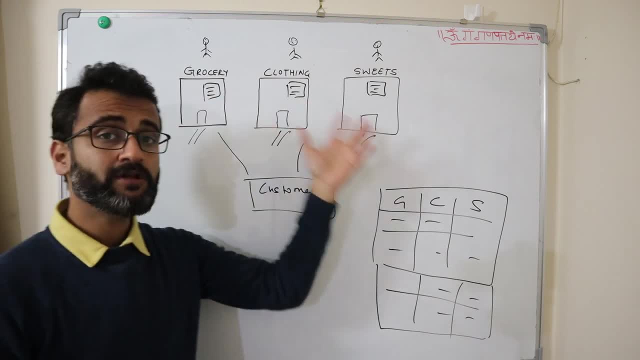 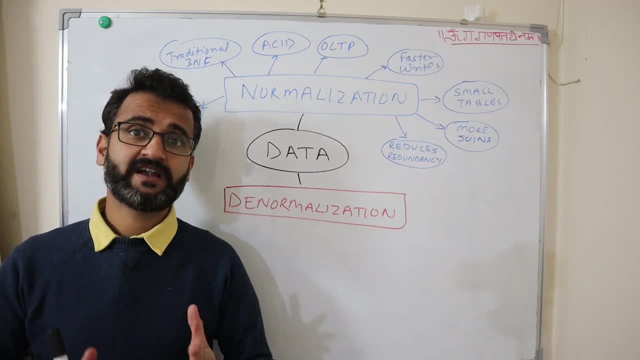 the details at one place, So they didn't have to look up all the different register, combine the data and you know the process of retrieving the data became very fast. So let's start with our understanding of normalization versus denormalization and specific features of these. 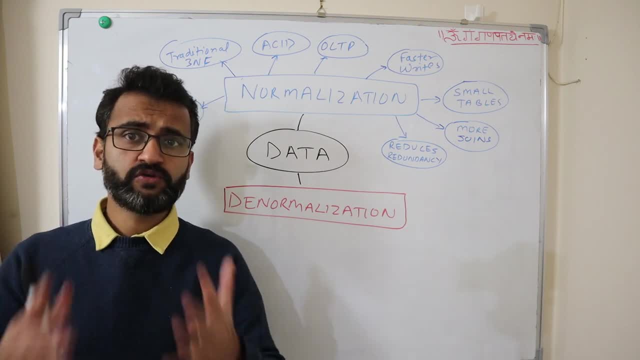 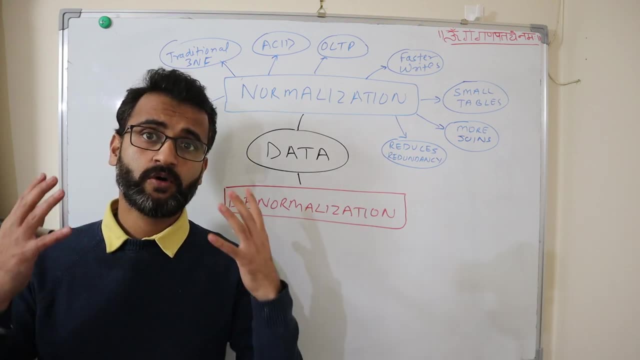 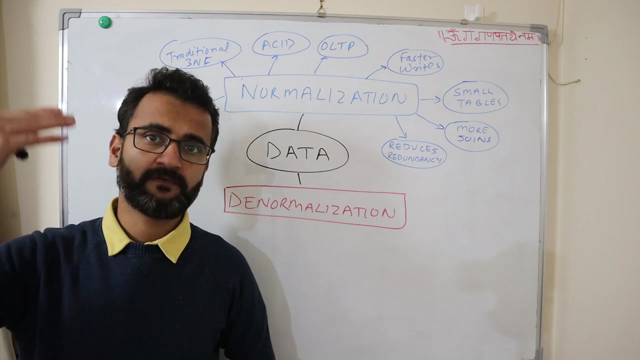 two techniques. So when we talk about normalization, it used to be- and it currently is- pretty much the traditional way of storing the data into a traditional OLTP system. and if you have heard the normalization technique, there are different degrees of normalization, like first normal form, second normal form, third normal form, and there are certain strict rules and regulations with. 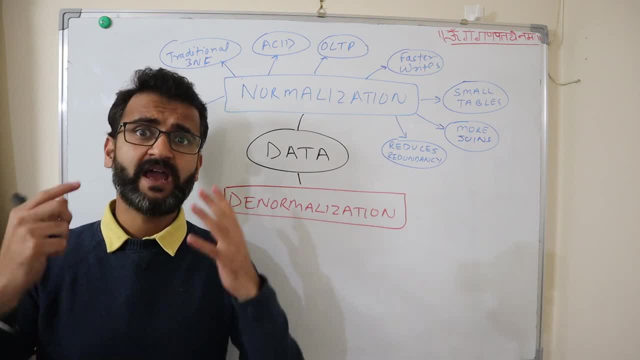 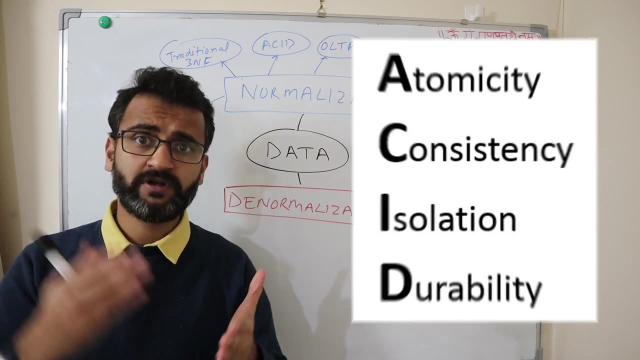 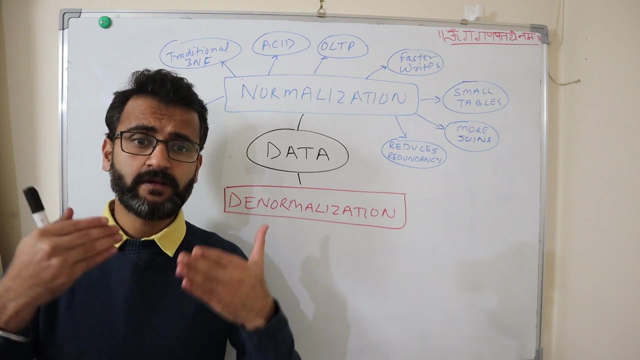 which you have to store the data, and that's why we have ACID compliant database, and these ACID compliant database ensures that we have no data redundancy. we have no redundancy, Data duplicacy or referential integrity is always in check, So these databases were made for very 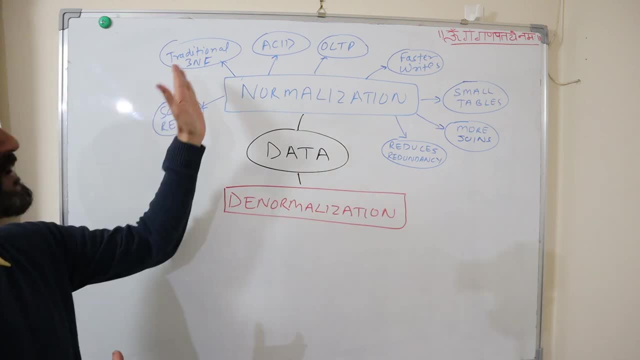 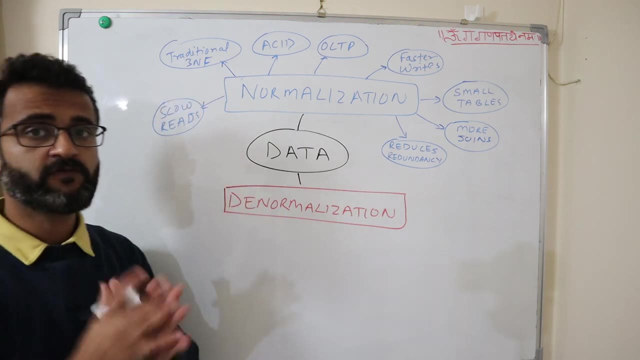 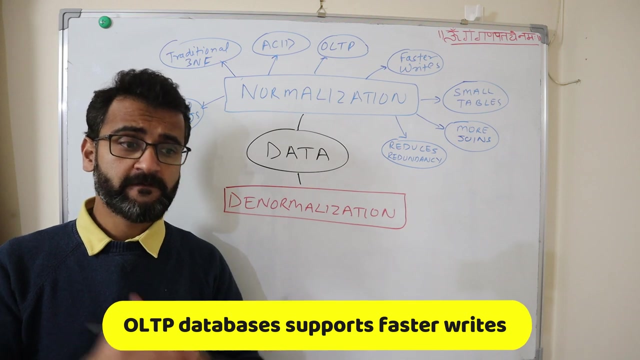 specific purposes of faster writes. So if you see it was a traditional third normal form. you know normalization techniques are generally applicable to traditional third normal form databases and it is generally for OLTP system which is used for transactional processing where we need heavy writes. So obviously what they will do in these 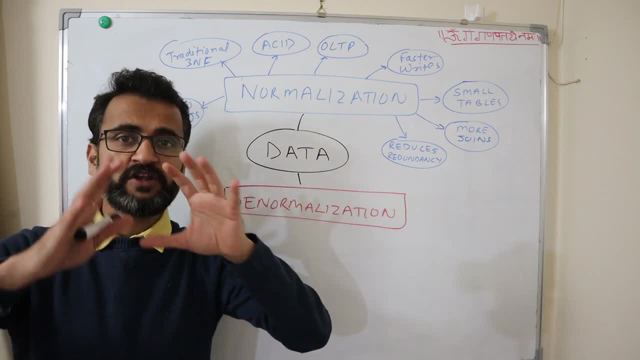 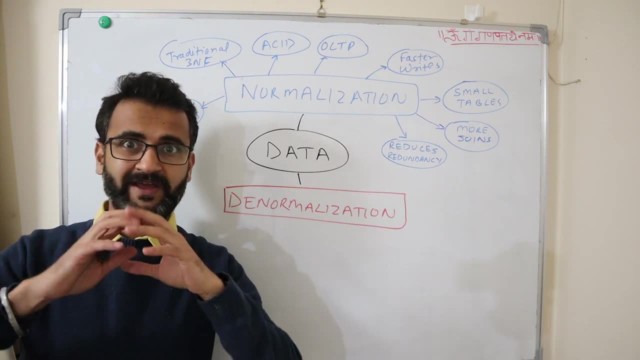 kinds of databases is that they will use the data duplication or referential integrity, which is what they call. The third kind of normalization technique is we will spread out our design into smaller tables and multiple joints, So you will have a very wide- you know- data model. very, very, very complex looking data model. 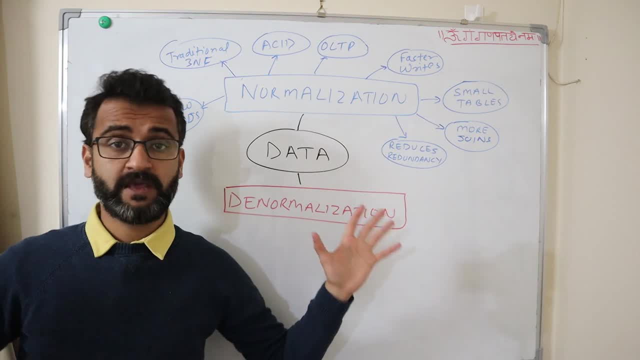 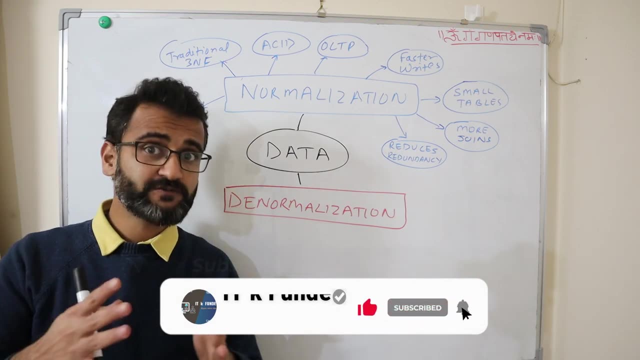 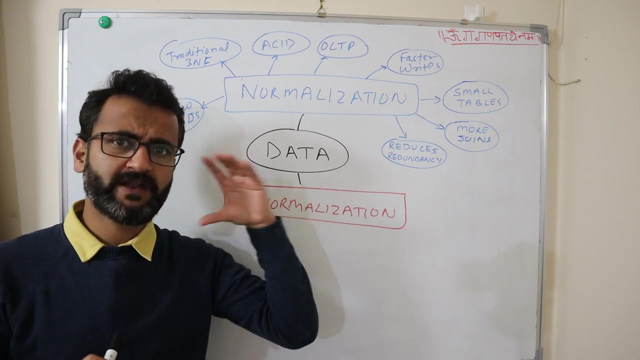 wherein you will have one table joining to multiple several tables and then whenever you want to fetch the data, you have to join it across all the tables. So that's why when you are writing the data into a normalized database, it's very fast. Take, for example: you have an employee table and if you are working, 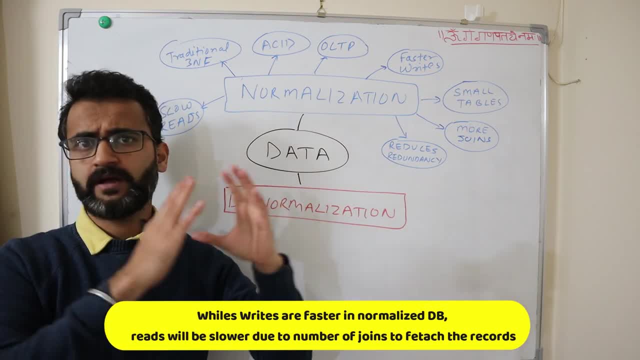 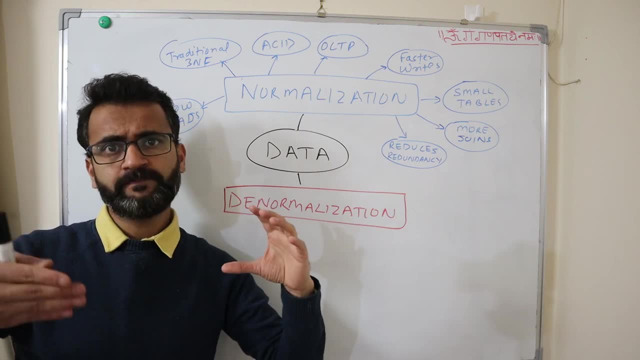 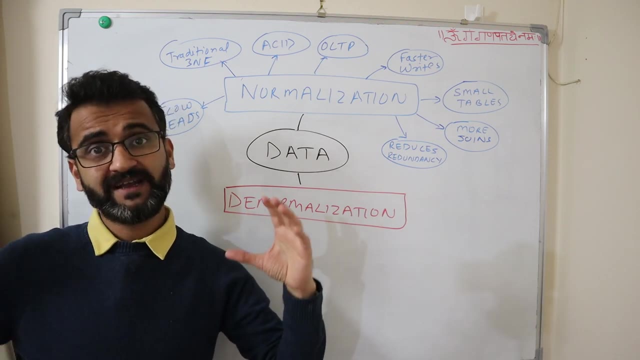 and you have a department table And then you have employee attributes, employee name, employee ID, salary, address, etc. And then you have a column, a key column, which is department ID, And then, using that department ID, you join it to a department table and get the department. 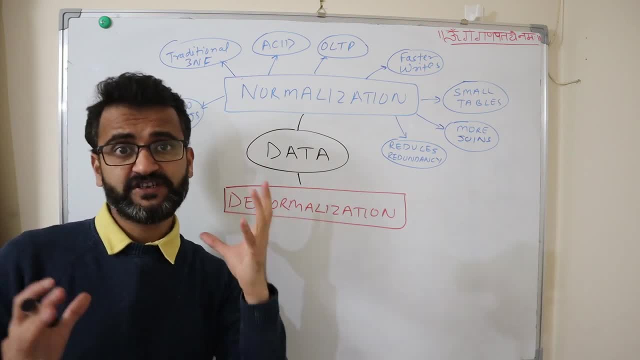 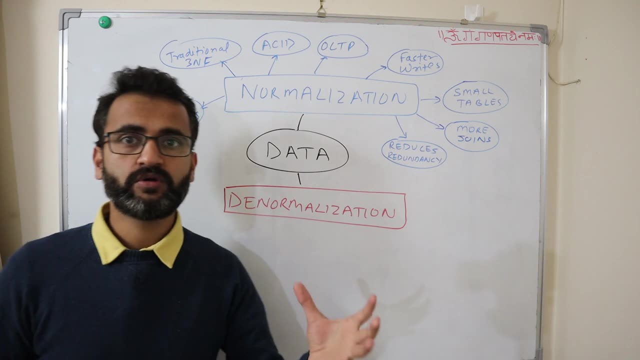 names from that particular table to understand which employee belongs to which department. So now, in this case, if you want to get the data, if you want to run the query, that okay, I want to understand which employee belongs to which department, then it has to join it. 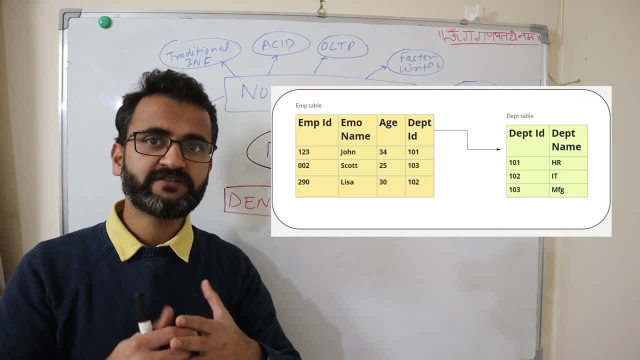 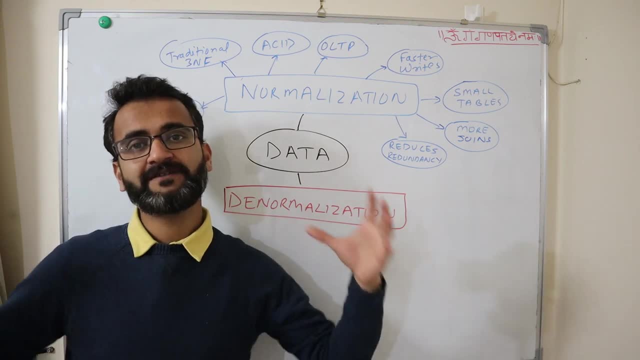 And sometimes the cost of joining is performance. If your joins are very complex and it is adding multiple tables into your query, it becomes very, very slow. So what if, instead of putting everything together, you bring the department name within the employee table? 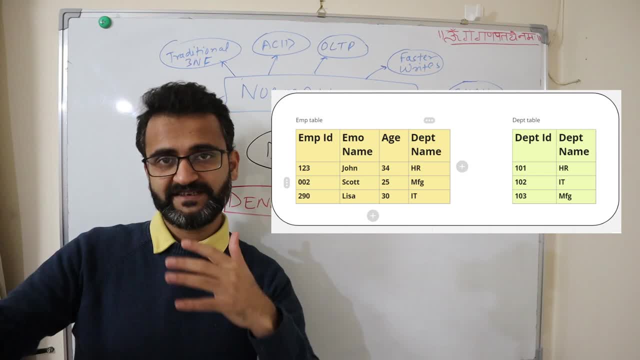 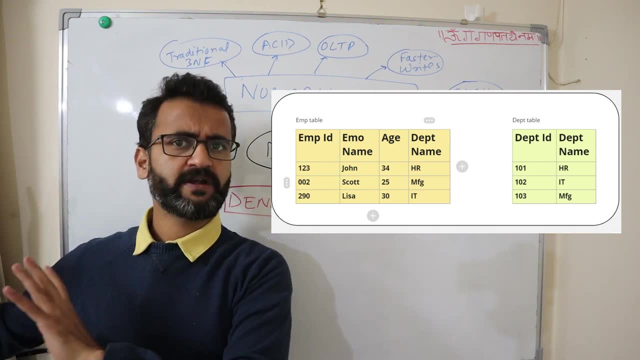 And then what you will have. you will, instead of running two different fetches from employee and department, you will have department name built inside the department name Inside the employee table And then you can have your separate department table to run and add additional attributes. 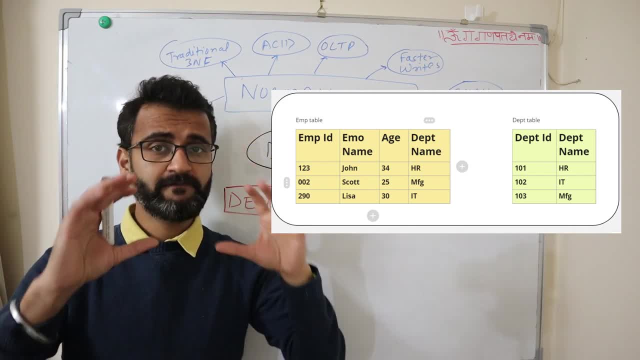 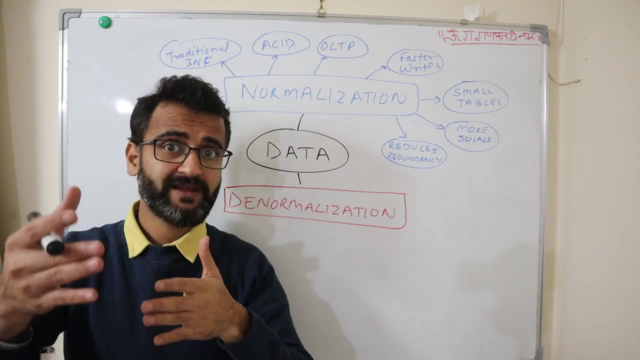 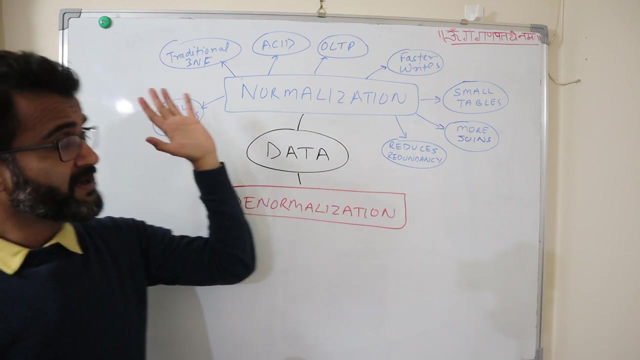 for department, But in this particular case your employee table will have that particular department name, So you can run the query exactly on that particular employee table. So that's where we denormalize the data, which we'll understand after this. So understand that it is good. 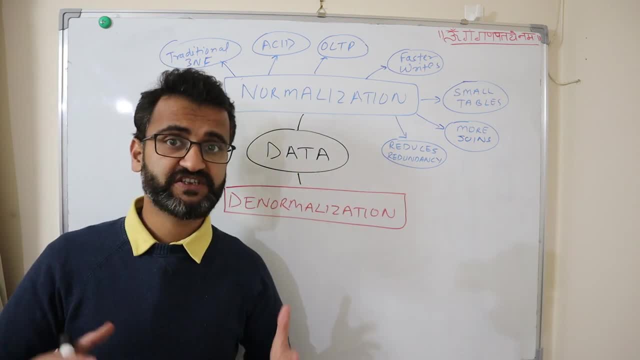 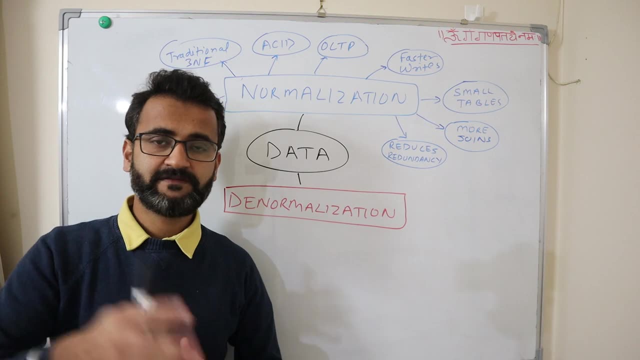 And it is good for certain cases where you have write heavy applications, where we have to focus on writing the data, Then you need to have a normalized database. So now let's understand the different features of denormalization. So denormalization, as we have discussed, works exactly in the opposite way. 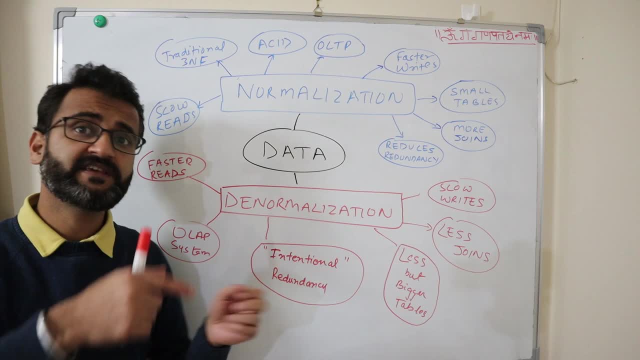 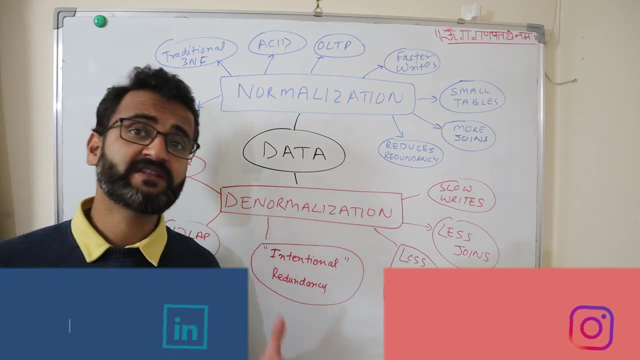 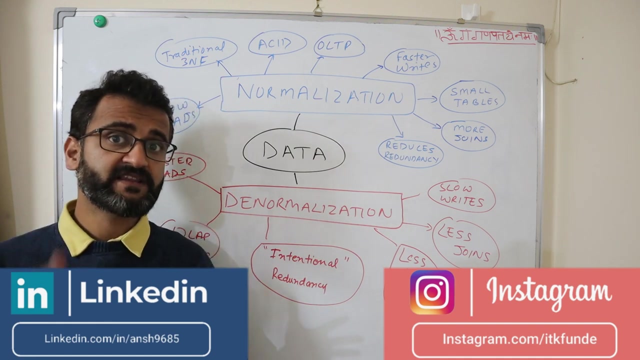 And it intentionally introduces redundancy into the data model, Because we want intentional duplication or redundancy so that we have everything in one plate and we directly get it from that particular plate, That particular table. Now, having said that, The caveat here Is that you cannot have, or you cannot afford to have, incorrect data. 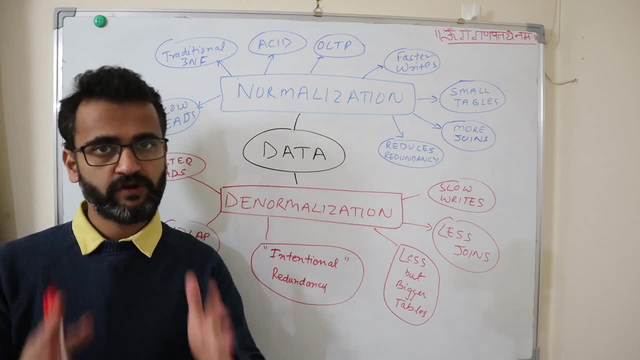 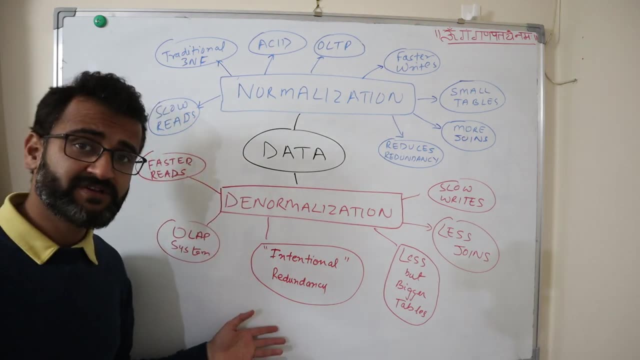 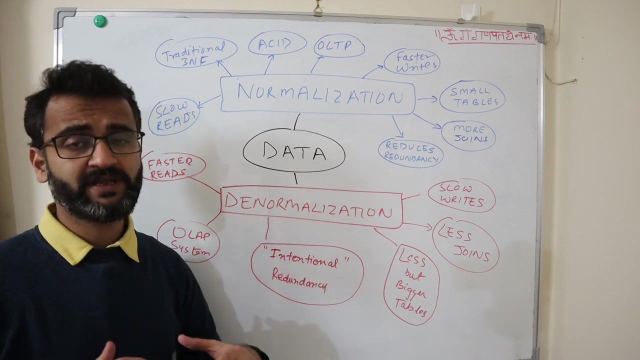 So, whichever technique we are using for data denormalization, we have to ensure that data correctness is intact. So it is exactly opposite to normalization. So it introduces redundancy. It has bigger, wider table. You know, in a denormalized data, you, you know you have a lot of data within, you know. 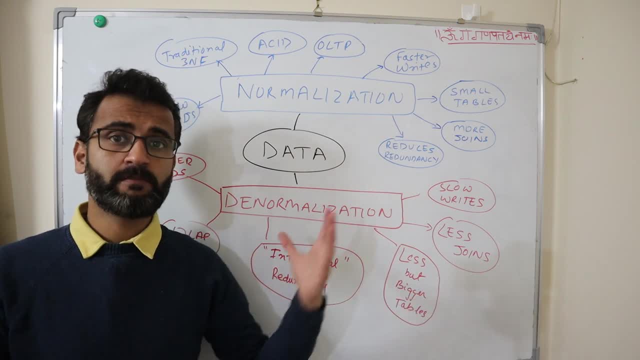 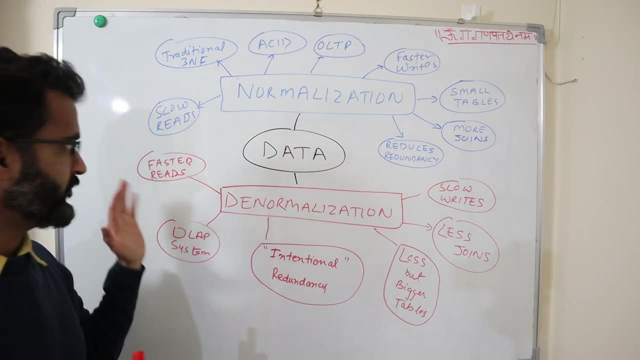 one particular table, Then you have obviously lesser joints, because if you combine everything in one table, then obviously your joints will get reduced And your performance will increase. So, on the flip side, while it will provide you with faster reads, when will it will come? 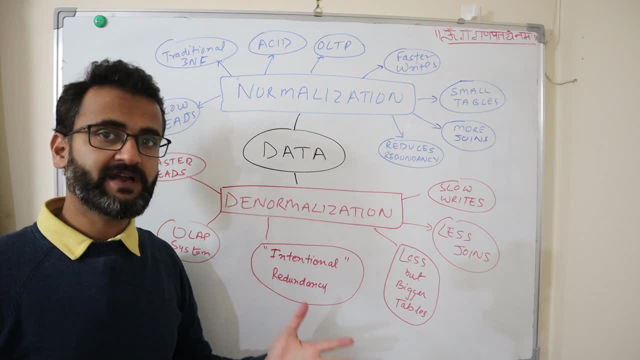 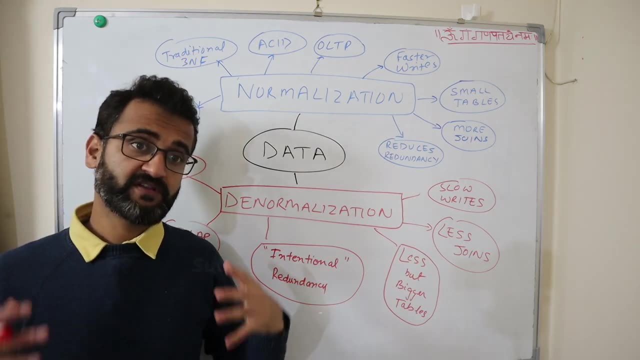 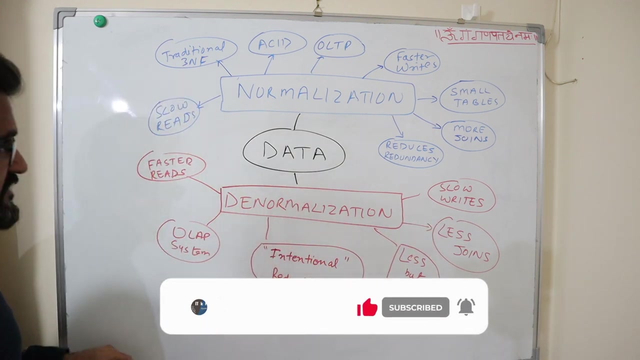 to writes, it would be slower than a normalized data Because, as we understand, we are, you know, putting everything in one particular table And we are making sure that the reads are faster, So writes will take a hit. One thing which I have missed in the comparison is that why we used to take normalization. 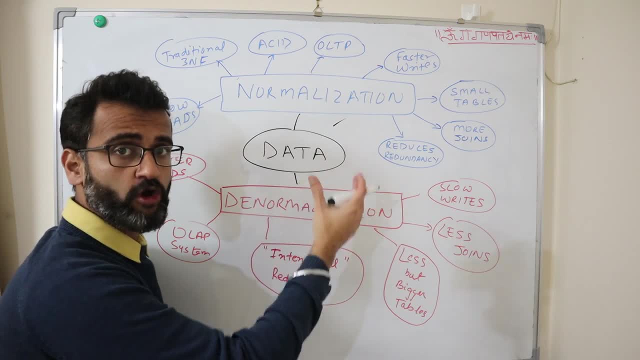 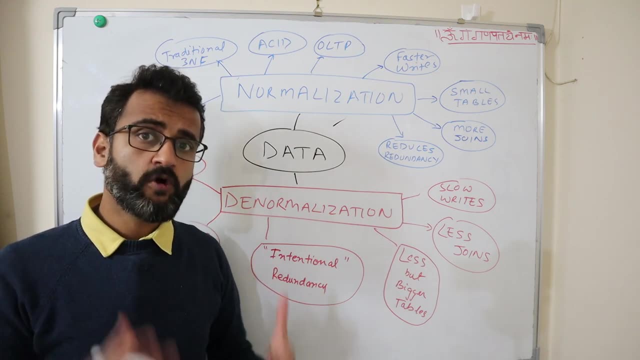 Why we used to take normalization, Why we used to take normalization, Why we used to give priority to normalization previously, was that in older times we had limited resources on the database, So we wanted to consume it very judiciously and very, very correctly. 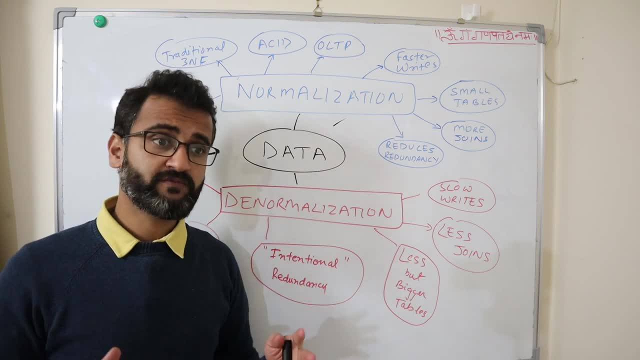 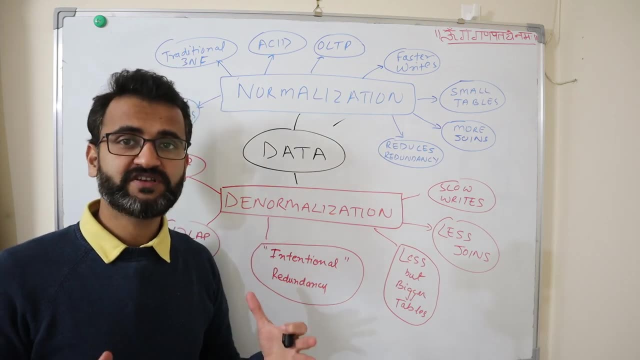 And that's why we used to take normalization And we used to ensure that whatever space we are using is, you know, adequate. But when the cloud computing came in, when we had very cheap resources available on cloud, we had no issues with denormalized data. Because the cost of queries were very, very cheap And instead of, you know, having those multiple joins and taking a lifetime to get the result, these cloud computing resources said: okay, you give me one particular table, dump everything in that particular table. I'm fine with, you know, some duplicacy. I'm fine with some null. 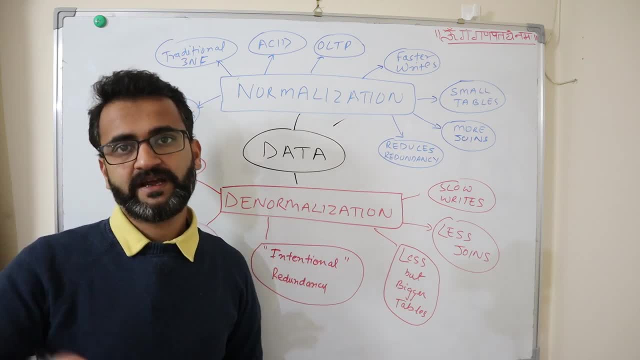 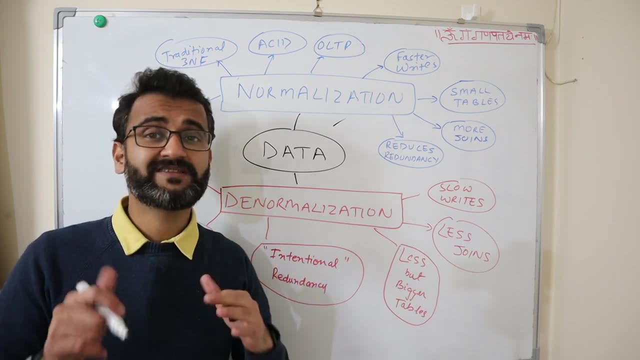 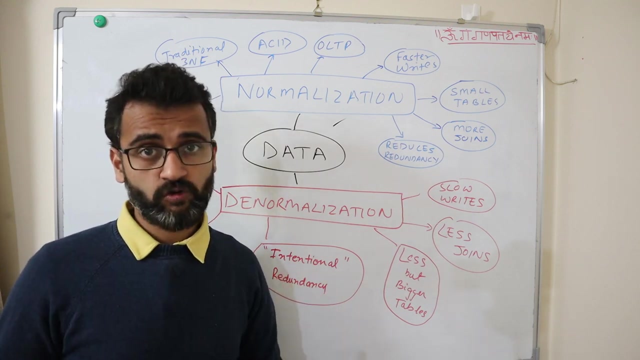 values, But if you give me one table, I'll make sure that I get you the results in seconds. So it actually wastes some resource. Denormalization wastes some resource, but then in a bigger context it is very minimal when we talk about the cost which we pay for a slower performance. 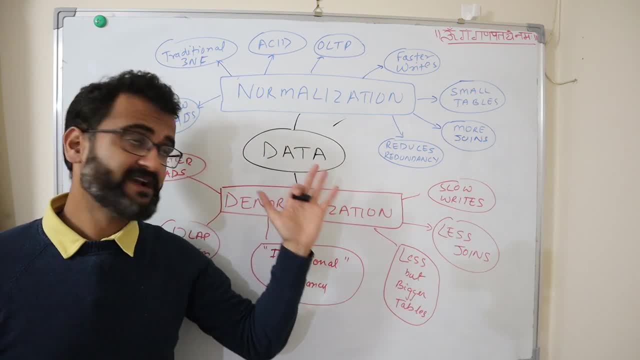 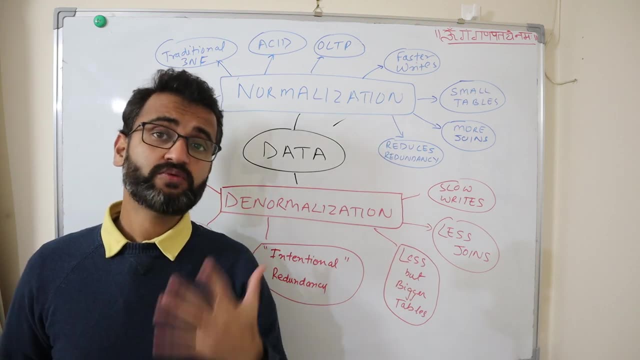 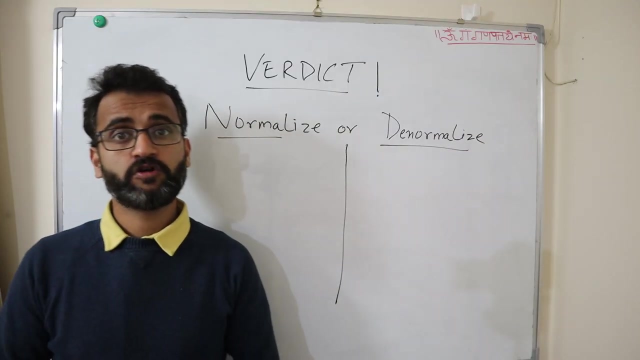 So, yeah, these are some, you know, some basic understanding of normalization versus denormalization. But the bigger question now arises: that which is better and when to choose what? So let's take that call now. So now, as we understand what is normalization, what is denormalization, 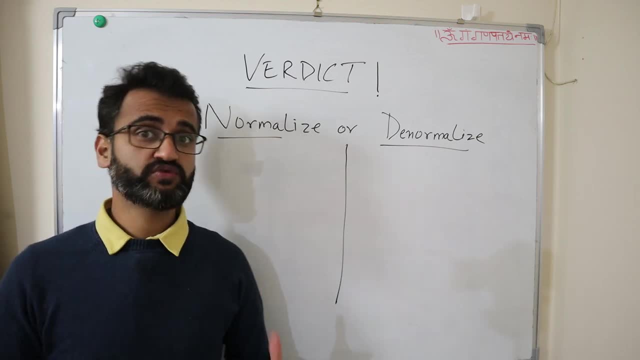 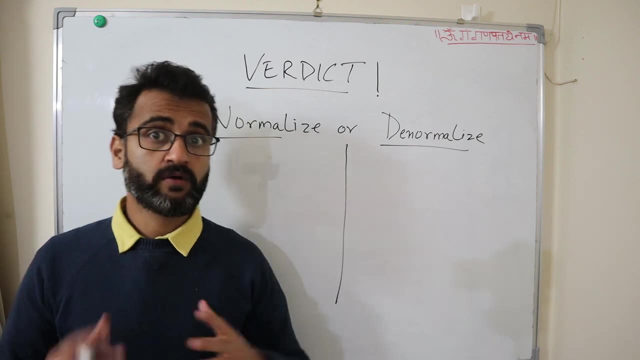 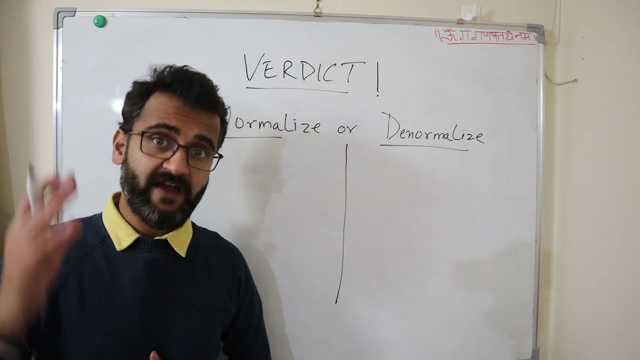 Here comes the interesting part of deciding and choosing which is better or which is not, or when to go for which particular technique. So in my perspective, both the techniques are good in its own sense And you, as a database architect or a data architect, have to decide in your particular. 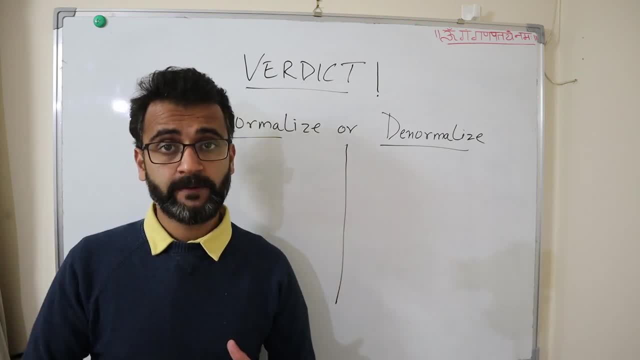 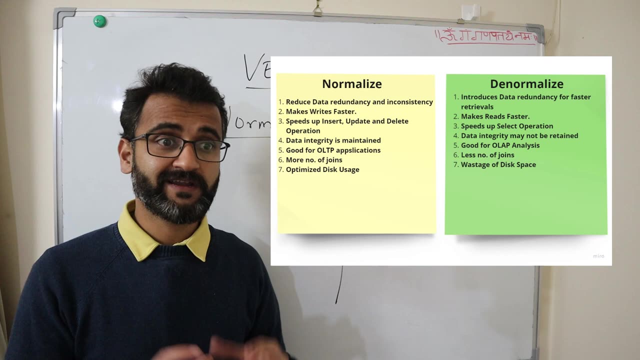 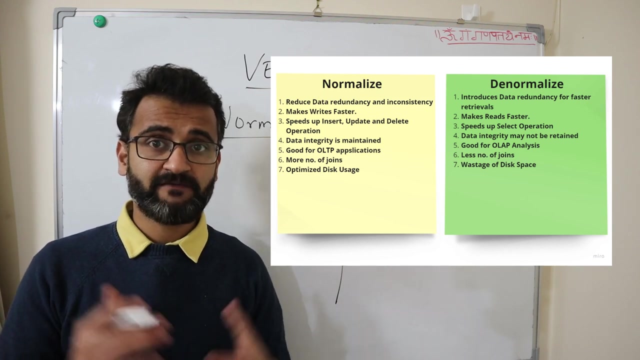 use case. which particular technique would be more useful If you are building a write heavy, intensive, write intensive application, suppose an ordering application. Let's say there are customers ordering something every two seconds, three seconds, every minute. Those kind of write heavy applications should have a normalized database or normalized data. 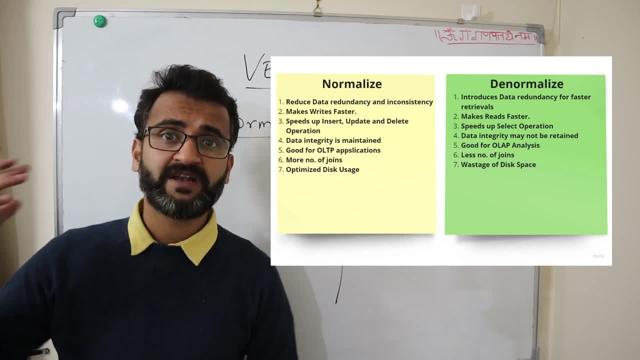 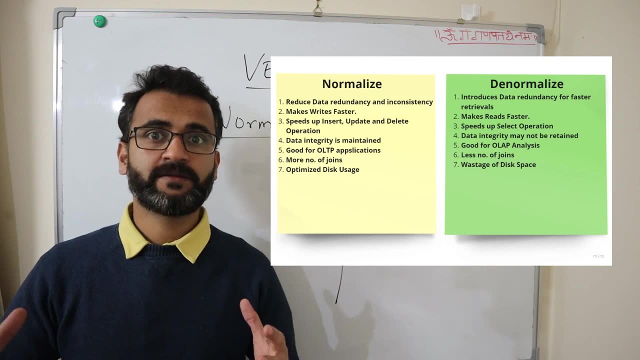 model, Whereas if you are building a data warehouse or a data lake solution where you have OLAP analysis, where you have BI reports, where you have, you know, trend analysis reports which you need to run, then in those cases you need to have denormalization. 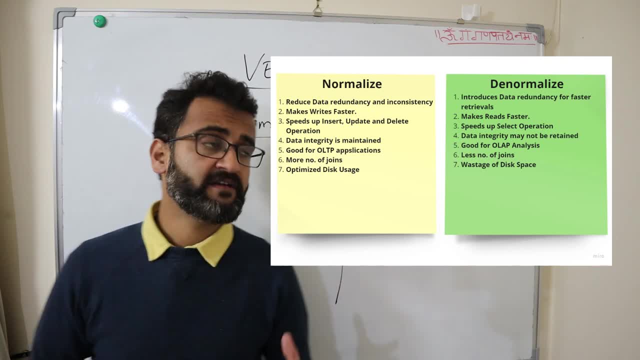 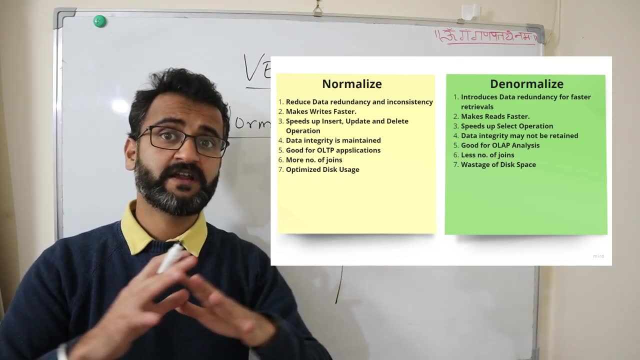 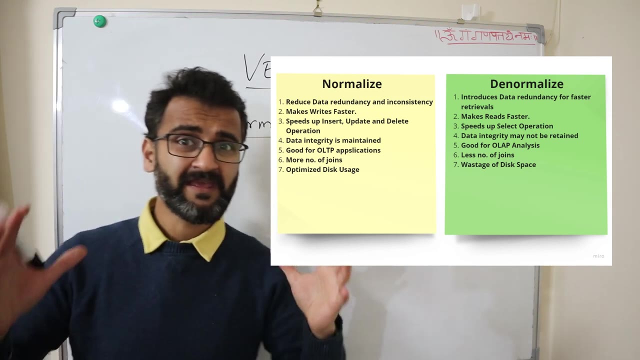 But at any given point of time It is not mandatory that you have to normalize to the nth degree and then, or or you have to denormalize the data completely. You can have best of both the worlds. So if we go back to our first layman example where we had three different shops, okay,